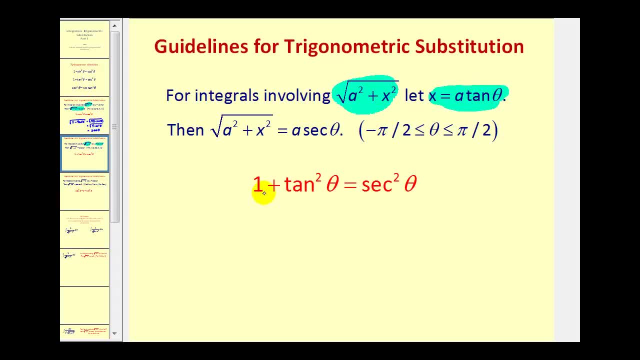 squared theta. If we use the identity one plus tangent squared theta equals secant squared theta. the square root of a squared plus x squared in this case will be equal to a secant theta. Then the last case will be when we have an integral involving the. 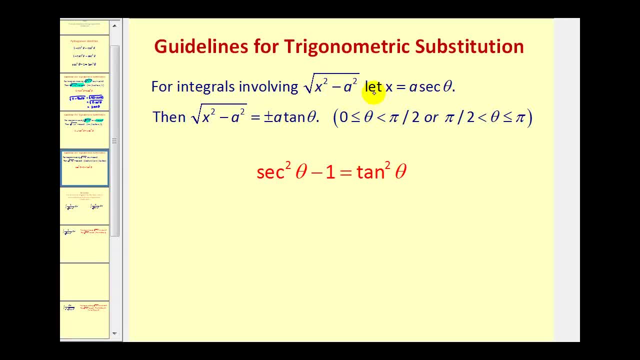 square root of x squared minus a squared, and in this case we'll let x equal a secant theta. Therefore, the square root of x squared minus a squared will equal plus or minus a tangent theta. Notice, this one has a plus or minus and that's based upon the angle theta Since tangent. 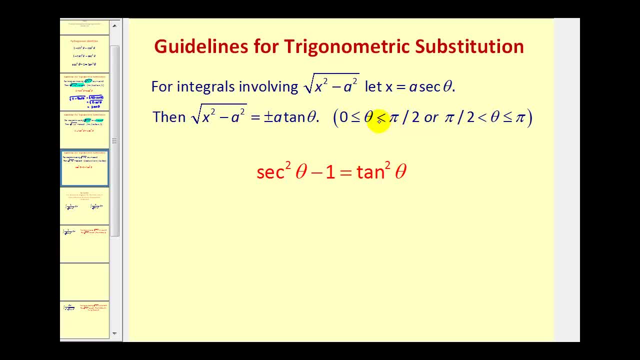 theta is positive. between zero and pi over two, we'd use positive a. and between pi over two and pi tangent theta is negative, so we'd use negative a Again. this equation here is based upon the fact that secant squared theta minus one is equal to tangent squared. 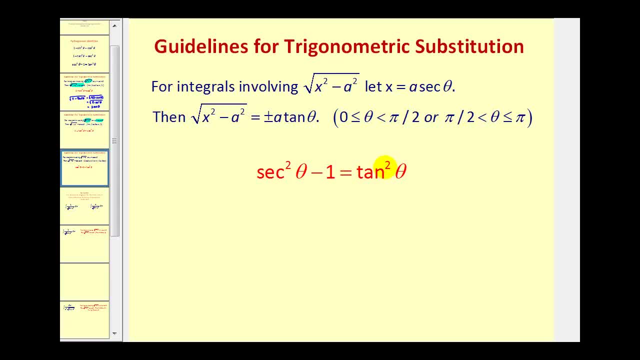 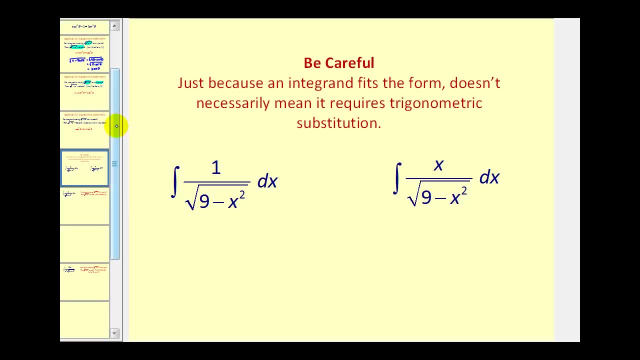 theta. One last word of caution before we take a look at our first example. We don't want to assume that every integral in the forms discussed will require tric substitution. For example, if we compare these two integrals, only one of them would require tric substitution: The. 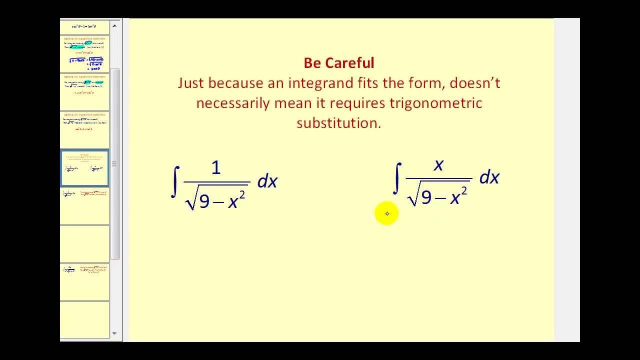 other one only requires basic u substitution. Can you recognize the one that requires basic u substitution? It's actually the second one here, because if we let u equal the radicand 9 minus x squared, then differential u is going to equal a negative 2x dx, which is: 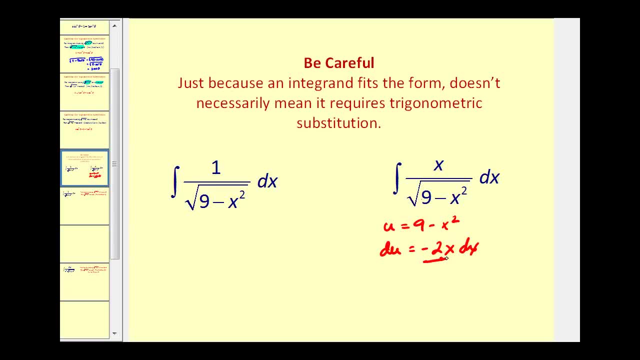 the integral of u. Notice, this integral does have x dx. so if we divide both sides by negative 2, we have negative one half du is equal to x dx. So we could rewrite this in terms of u. What we would have is, again, x dx would equal negative one half du, and this would 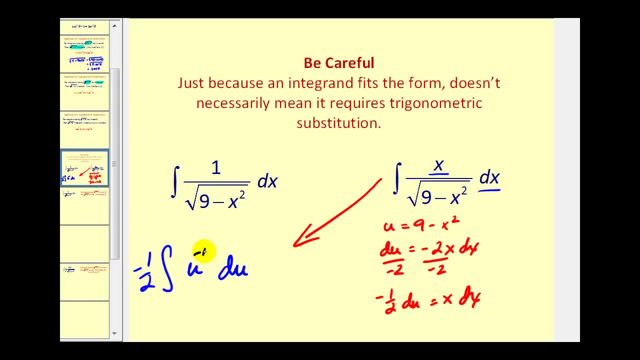 be one over the square root of u or u to the negative one half. So we could find the antiderivative using basic u substitution. However, on this integral we would have to use tric substitution. Let's go ahead and take a look at our first example. Notice: the integral involves the 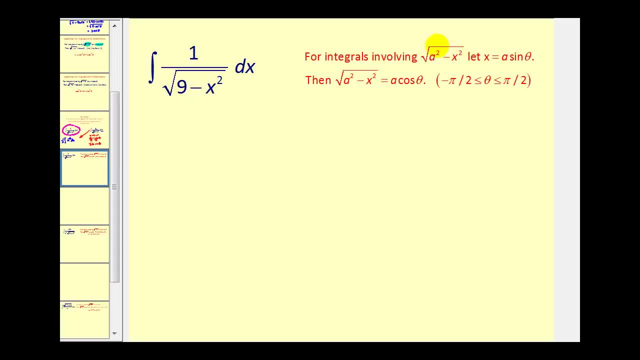 square root of 9 minus x squared. So this involves the form: the square root of a squared minus x squared. So a squared is going to equal 9, therefore a would be equal to 3.. So we're going to let x equal 3 sine theta. 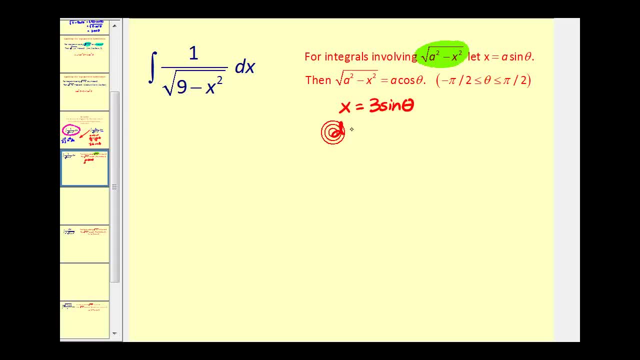 Now let's go ahead and find differential x. Differential x is going to equal 3 cosine theta, d, theta. Now the last thing we need to do before we perform this substitution is sketch a triangle that represents angle theta. We're going to need that toward the end of 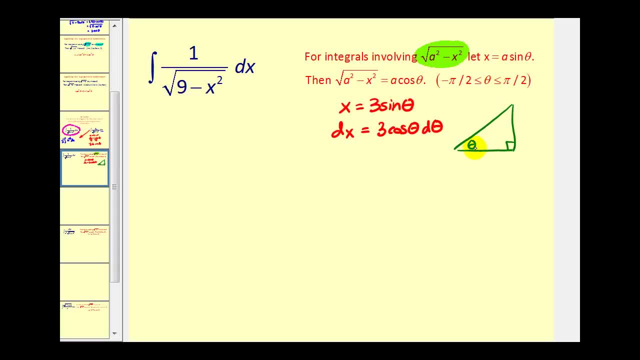 the problem. So let's sketch a right triangle identifying theta. Now we can get this equation here and if we solve this for sine theta, sine theta will be equal x over 3, which would mean the opposite side would be x. 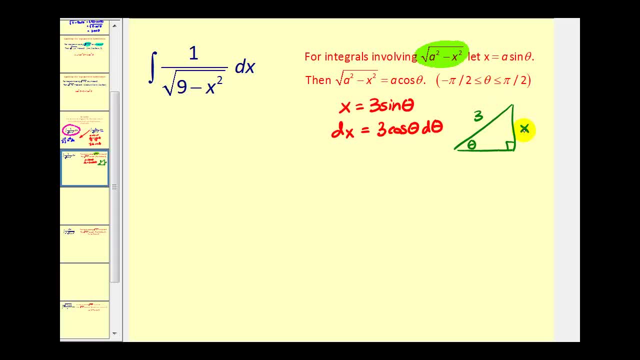 and the hypotenuse would be three. So using the Pythagorean theorem we could state that this side here would be the square root of three squared minus x squared, or nine minus x squared. Now let's go back to the integral and perform the substitution. 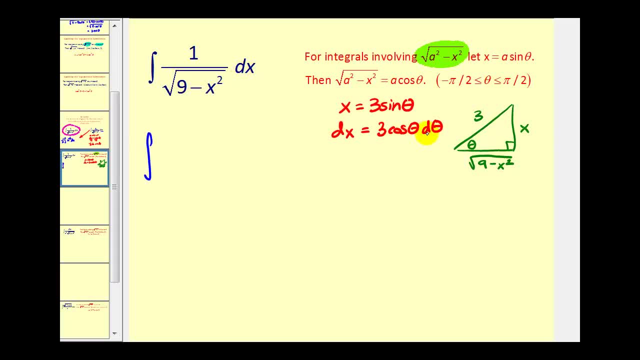 Notice that dx is equal to three cosine theta d theta. So we'll have three cosine theta d theta over the square root of nine minus x squared Well, that would be nine minus nine sine squared theta. Now, performing this substitution, this denominator is going to simplify nicely. 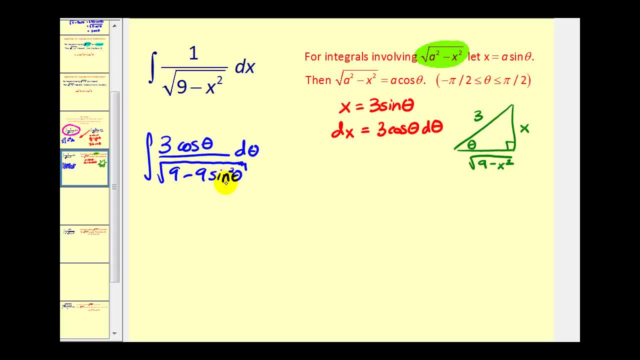 Remember the square root of nine minus nine sine squared theta simplifies nicely to three cosine theta. So this is equal to three cosine theta over three cosine theta d theta. Well, of course this simplifies to one And the anti-derivative of one with respect to theta. 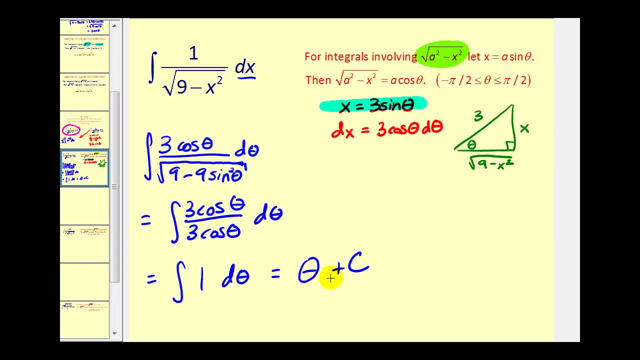 would be theta plus c. So we do have the anti-derivative here, but it's not in terms of x like the original integral. So we can't leave our answer in terms of theta, And that's why it's so important that we have this right triangle here. 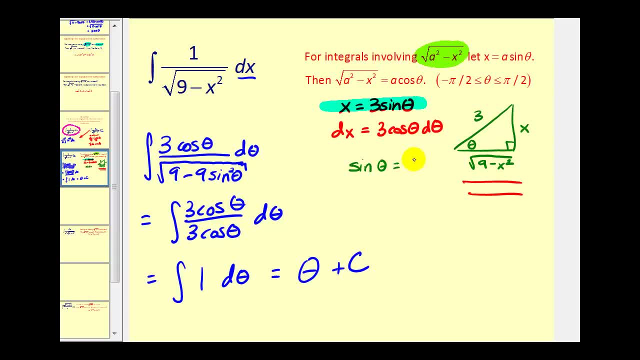 We know that sine theta is equal to x over three. So if we take the inverse sine on both sides, we can solve this equation for theta in terms of x, to express our anti-derivative in terms of x. Remember the inverse sine of sine theta. 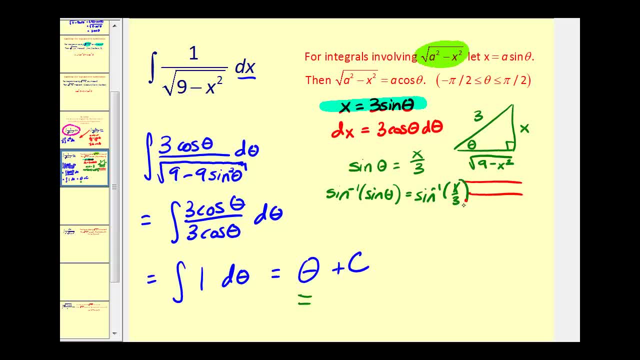 equals the inverse sine of x over three. On the left we have inverse sine of x over three. Therefore the anti-derivative in terms of x will be inverse sine x over three plus c. So it is very important that we remember. 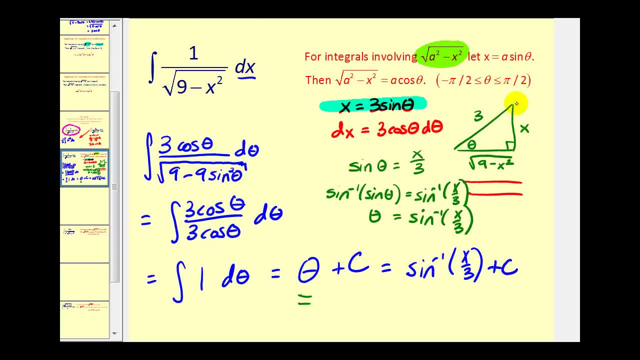 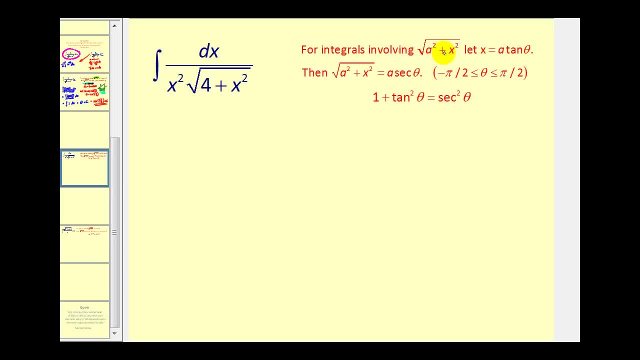 when we're setting up this integral from the beginning, that we do sketch a right triangle that models our angle theta. Okay, this is going to be the end of part one. In the next video, we'll take a look at the form. 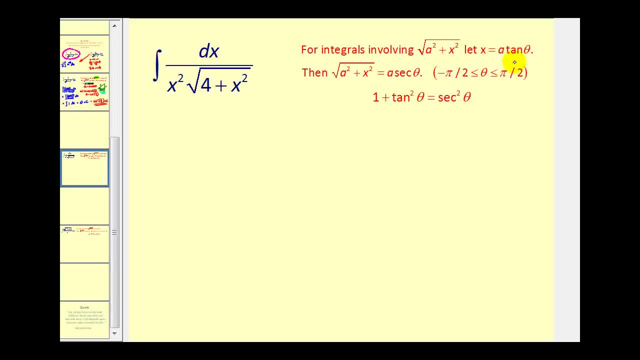 of the square root of a squared plus x squared when we let x equal a tangent theta. I hope you watch part two. 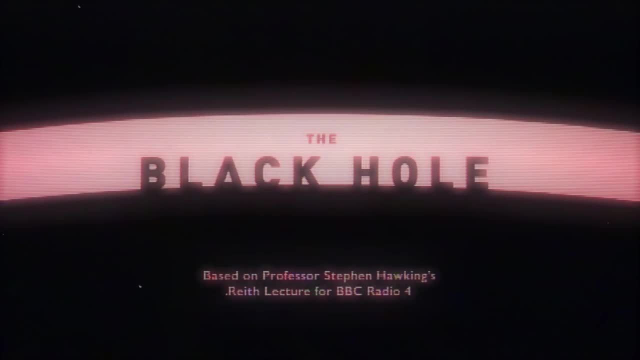 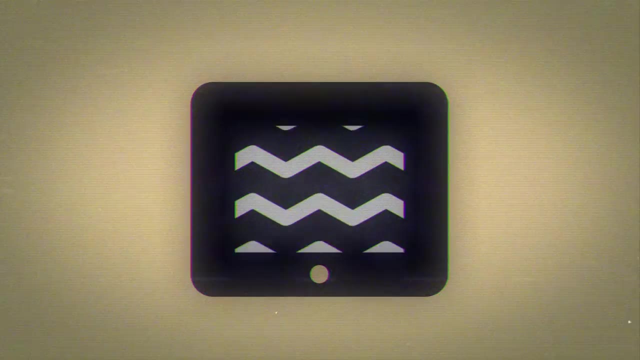 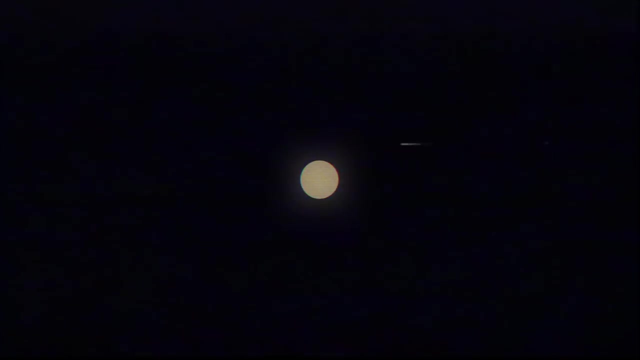 From the outside you can't tell what is inside a black hole. You can throw television sets, diamond rings or even your worst enemies into a black hole and all the black hole will remember is the total mass and the singular momentum and electric charge. Quantum mechanics. 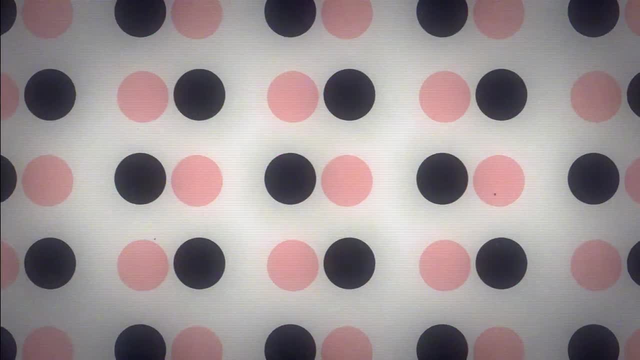 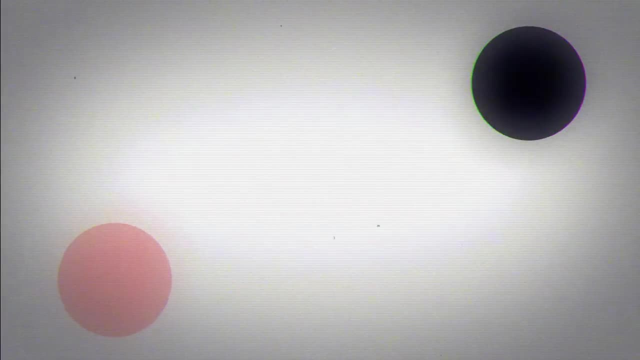 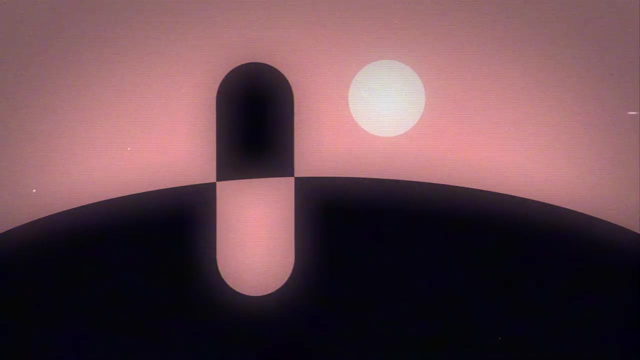 implies that the whole of space is filled with pairs of virtual particles and antiparticles that are constantly materializing in pairs and then coming together again and annihilating each other. One member of a pair of virtual particles may fall into the hole leaving. 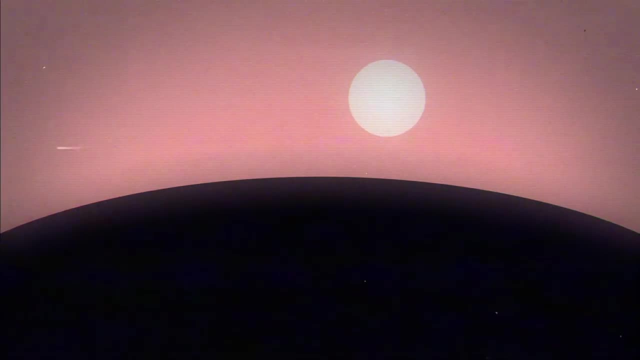 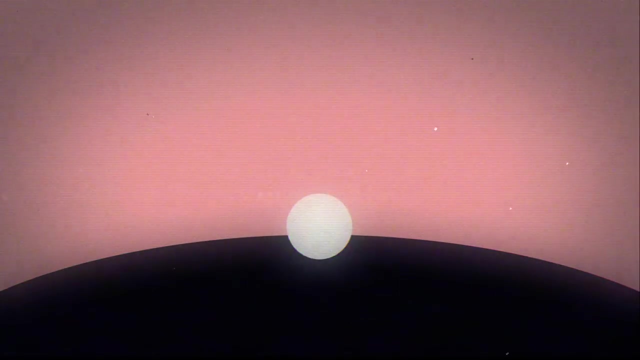 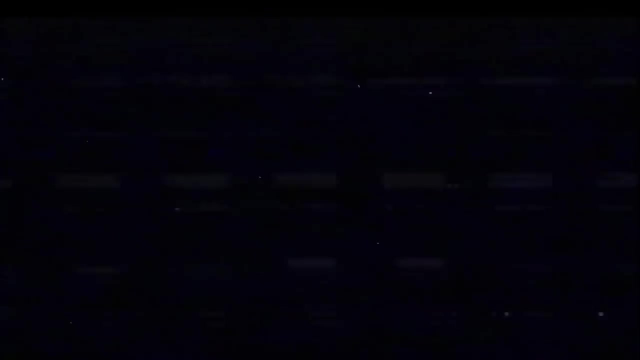 the other member. without a partner with which to annihilate, The forsaken particle or antiparticle may fall into the black hole after its partner, but it may also escape to infinity, where it appears to be radiation emitted by the black hole. The message of the black hole is that the black hole is a black hole. 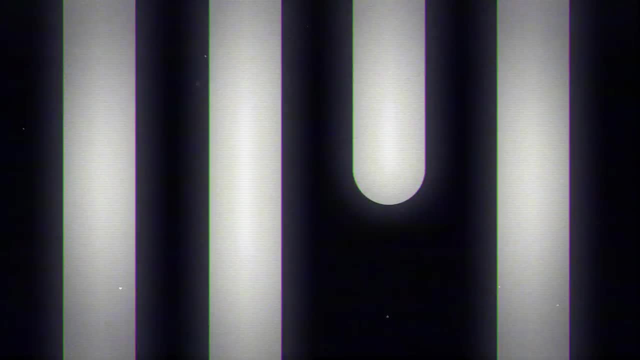 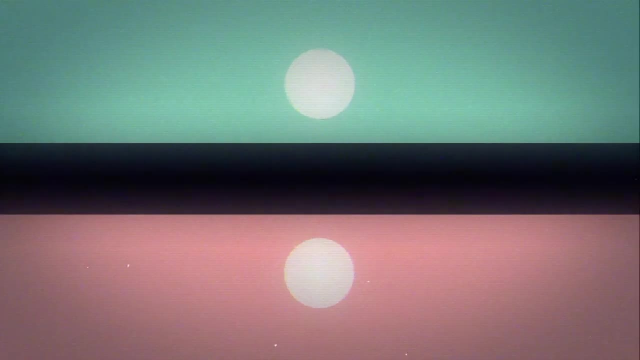 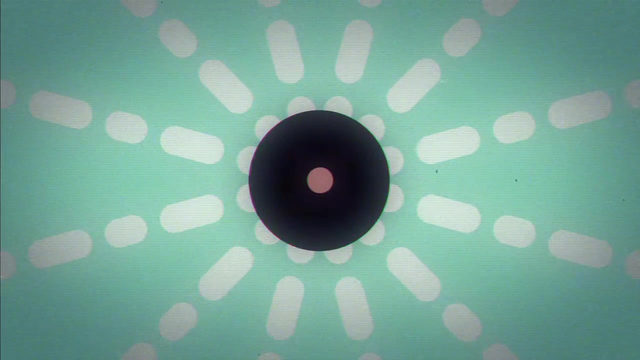 This lecture is that black holes ain't as black as they are painted. They are not the eternal prisons they were once thought. Things can get out of a black hole, both to the outside and possibly to another universe. So if you feel you are in a black hole, don't give up. 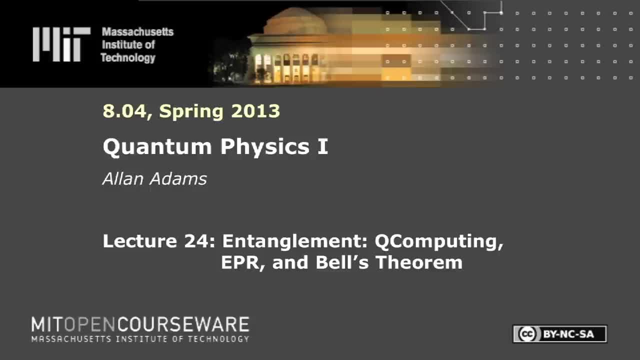 The following content is provided under a Creative Commons license. Your support will help MIT OpenCourseWare continue to offer high-quality educational resources for free. To make a donation or to view additional materials from hundreds of MIT courses, visit MIT OpenCourseWare at ocwmitedu.